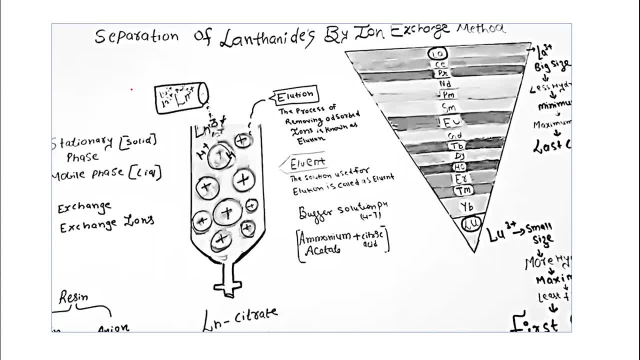 This is the resin column. we require cation exchange resin column. here. We require cation exchange resin column, Cation exchange- Lanthanone ions are cation, so they are going to exchange. So this cation exchange resin column, it is a solid phase. 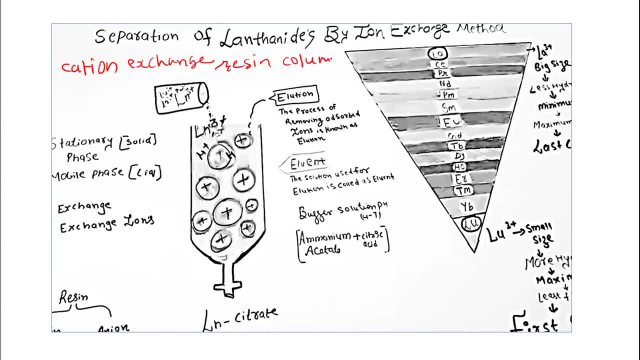 or stationary phase. in chromatography we are using the two phases, stationary phase and mobile phase, in any type of the chromatography. okay, this is adsorption chromatography. so in this case, the stationary phase, which is a solid phase. it is a cation exchange regime column. 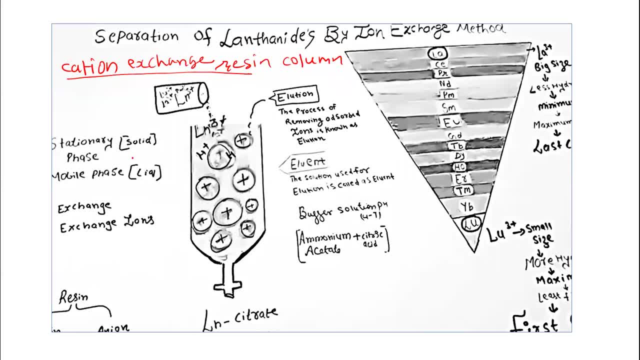 which contain the cation and the mobile phase. it is a liquid here, mobile phase. we are adding the mobile phase here during the separation of the lanthanum. first we have to prepare the resin column. okay, so this is a particular type of the burette where we can. 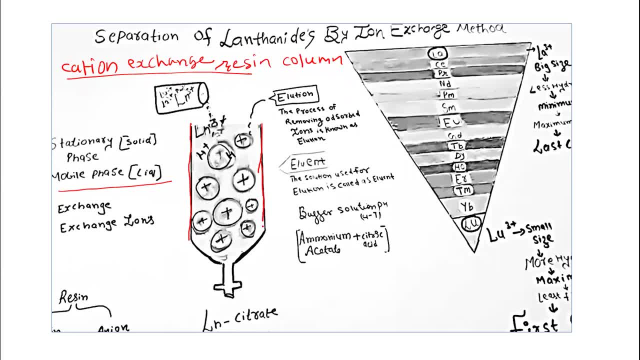 prepare the resin column. uh, take the cation exchange region column here. okay, we can take the cation exchange resin column here, so you can see this positive. it is shown here. this is a cation exchange region column, or it is represented as hr solid. okay, hr solid hydrogen ions are attached to this resin column, okay, 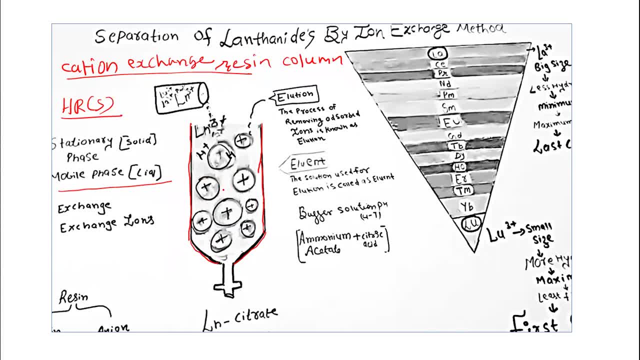 now, once we prepare the column. the most important thing in the ion exchange method is that we have to prepare the cation exchange region column. uh, there should be no any gap in the resin column. okay, it should be continuous. and later on, once the column has been prepared, then we should have to add: 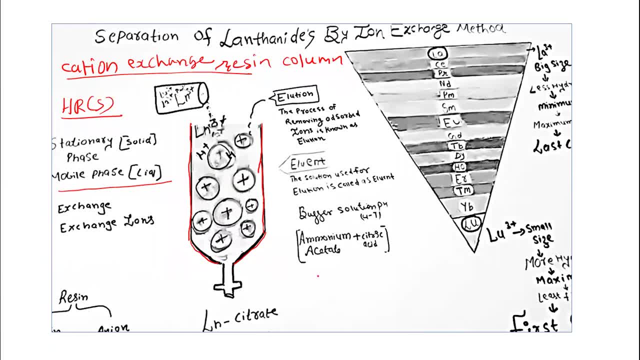 the solution of the lanthanons: aqueous solution of the lanthanon in the resin column or acidic solution of the lanthanon in the resin column. so what happens here? the lanthanon ions get attached to the resin column because it is a exsorption chromatography. so in exsorption chromatography, the chromatographyron. 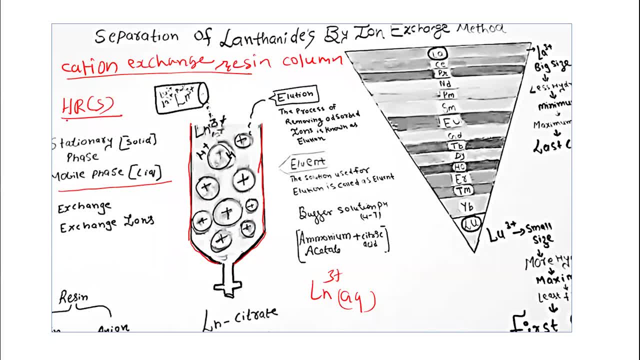 cartography. the cations get absorbed onto the resin column, get absorbed onto the solid resin. this is a solid resin and when we are adding this solution here in the resin column, the lanthanone ions are get attached to the resin column. okay, one by one, they are going to be attached with. 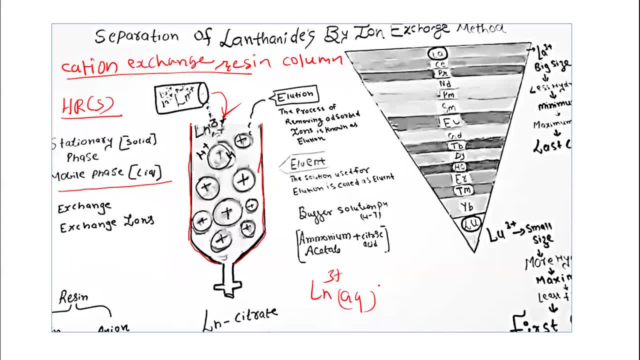 the resin column. let us show that process. so lanthanone ions get attached to the resin column. so ion exchange process is takes place here. ion exchange process is takes place here and equilibria has been established. so let us show this process: the lanthanone ions get. 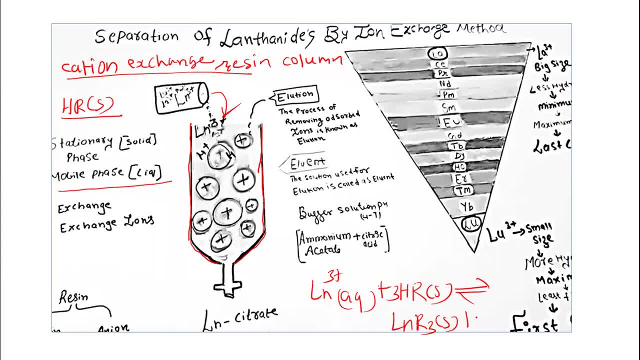 attached to the resin column. okay, and hydrogen ions now free from the resin. so when we are adding the equimolar solution of lanthanone ions in the resin column, the lanthanone ions get attached to the resin column one by one and the lanthanone ions are separated from each other. the lanthanone ions are separated from each other. 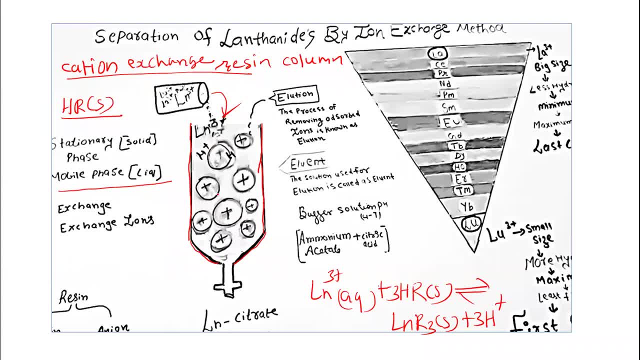 once again, i would like to tell how the process has been takes place. first of all, we have to prepare the resin column. okay, once the resin column is ready for the separation, then we have to add the solution of the lanthanone ion in the resin column. 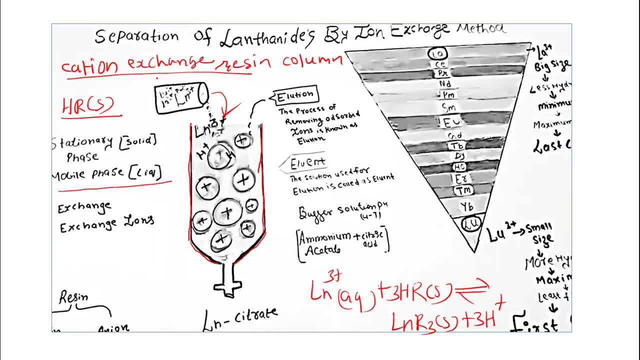 we have to pour the solution of the lanthanone ion in the resin column. okay, aqueous solution of the lanthanone ion in the resin column. so, due to the addition of the aqueous solution or acidic solution of the lanthanone ion in the resin column, 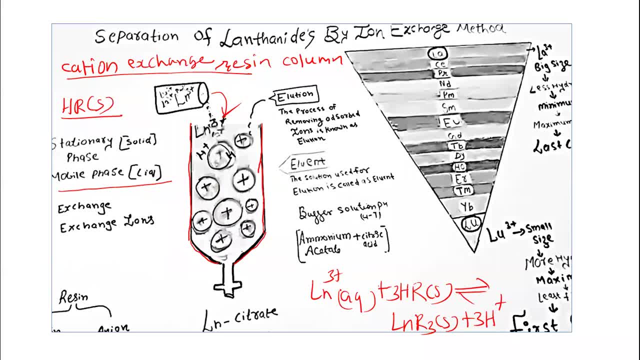 aqueous solution or acidic solution of the lanthanone ion in the resin column. the lanthanone ions get exchanged with the resin one by one, not simultaneously one by one. they are going to exchange with the region and the lanthanone ions are binds with the resin column, so they are going. 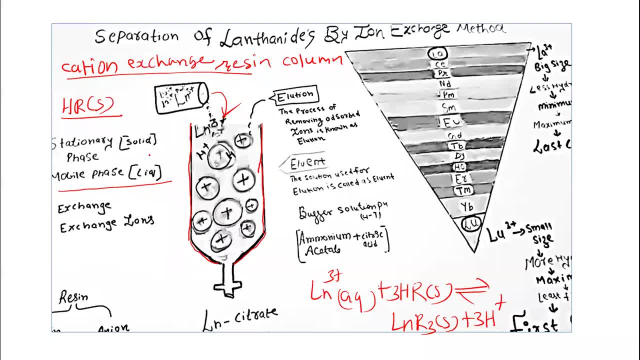 supposed to be in the stationary phase and hydrogen ions are free here. now they are going into the mobile phase. initially, hydrogen ions are attached to the resin column because it is a cation exchange region column. hydrogen ion is a cation, so there is an exchange between lanthanone ions and hydrogen ions is takes place. okay, and this exchange process. 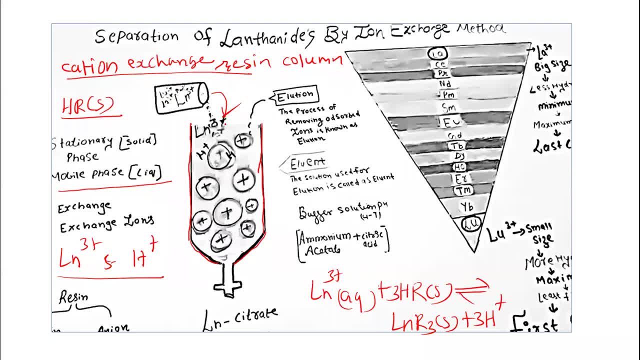 it is takes place when we are adding the solution of the lanthanone ions in the resin column. so, one by one, the lanthanone ions get exchanged with the resin column. now the question is that which one lanthanone ion is exchanged first? so what is the principle involved in? 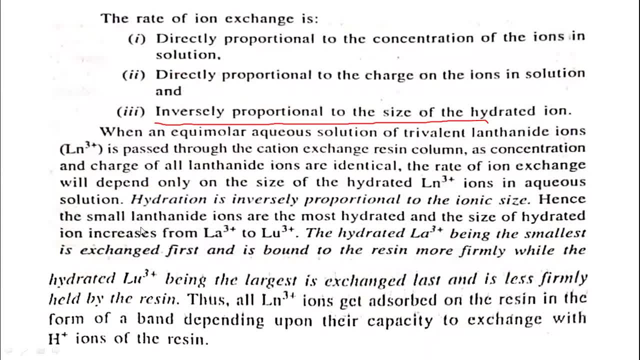 the separation of the lanthanone. so let us see: there are three principles mainly included here. first of all, the rate of the ion exchange is directly proportional to the concentration of the ions in the solution. second, the rate of the ion exchange is directly proportional to the concentration of the ions in the solution. second, the rate of the ion exchange is directly 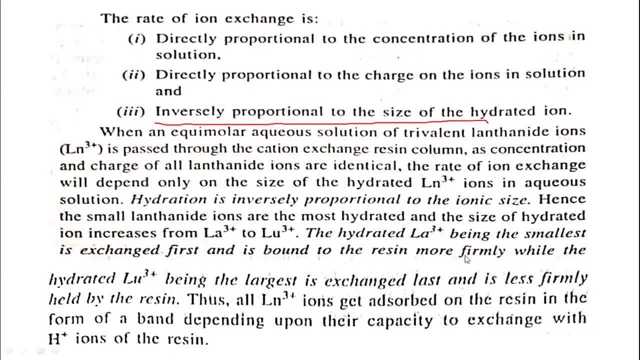 proportional to the charge on the ions in the solution. and third, the rate of the ion exchange is inversely proportional to the size of the hydrogen ion. so in this case the first two principles are same for all the lanthanone ions. from this we cannot differentiate. 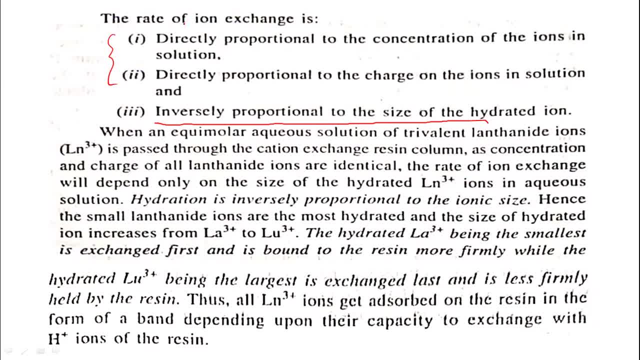 in the rate of the ion exchange. we cannot differentiate in the things you see here as shown on this slide. then then for theoner application, we cannot differentiate between times and Jenna. if I tried to multiply the number of Celsius and let us say one whole, the rate of the ion exchange. okay, so rate of the ion exchange is directly proportional to. 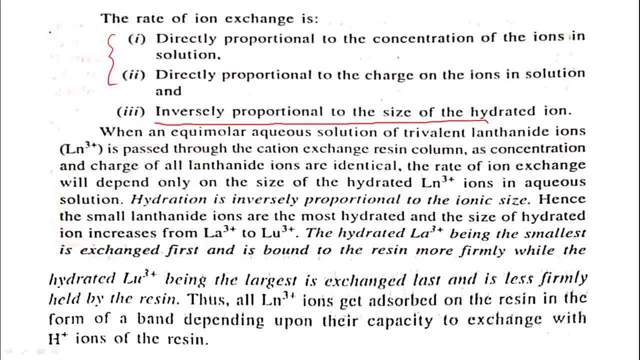 the concentration of the lanthanum ions. we know that all the lanthanum ions are having the equimolar concentration. equimolar concentration because they are present into the same solution. so they are having the equimolar concentration means their concentration it is same equimolar concentration. 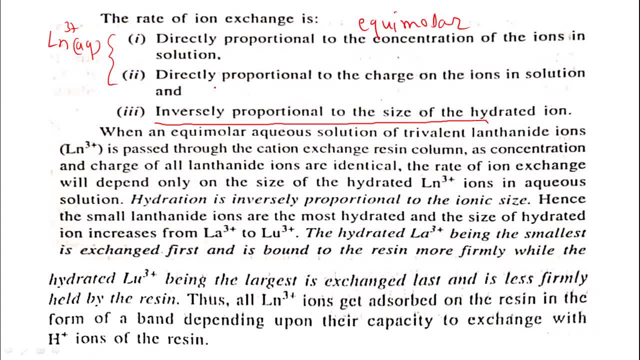 okay then the rate of the ion exchange is directly proportional to the charge on the ion. second principle: but as we know, all the lanthanum ions are having the tripositive oxidation state, so their charge will be same. so rate of the ion exchange is same for all the lanthanum ions. 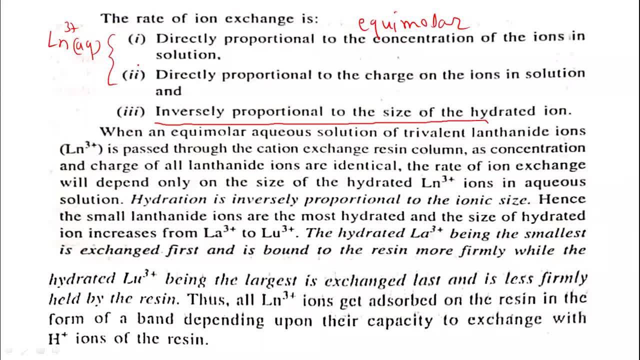 okay, these two principles are same for all the lanthanum ions. now this is now third principle: rate of the ion exchange is inversely proportional to the size of the hydrated ion. size of the hydrated ion. so, with the help of this principle, we can explain which one lanthanum ion is exchanged first with the resin column. 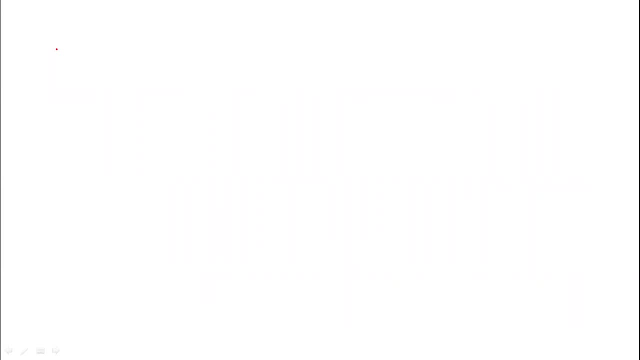 okay. so let us write down this principle now. so rate of the ion exchange, rate of ion exchange is inversely proportional. rate of the ion exchange is inversely proportional to the size of the hydrated ion. size of hydrated ion: okay. size of hydrated ion, hydrated radius: okay. it means that those lanthanum ions who are having smaller hydrated radius 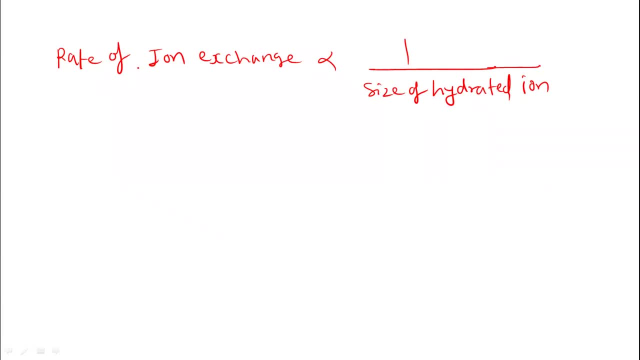 the rate of the ion exchange will be greater. those lanthanum ions. lanthanum ions who are having smaller or smallest smallest hydrated radius. smallest hydrated radius: the rate of the ion exchange is greater for that. lanthanum ions: the rate of ion exchange is greater for that lanthanum ions. 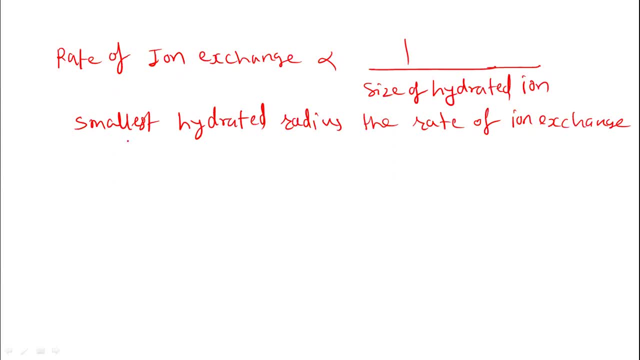 so which lanthanum ions are having the smallest hydrated radius? now, in this case, there is a one important thing: hydration is inversely proportional to the ionic size. hydration is inversely proportional to the ionic size. okay, it means the lanthanum ions which. 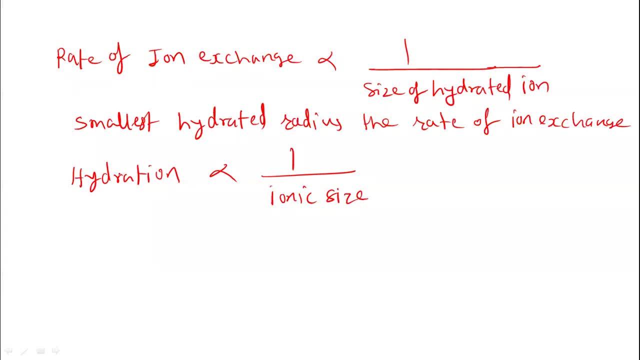 are having the smaller ionic size. they are mostly hydrated and they are hydrated radius will be largest. the lanthanum ions who are having the smallest ionic size. so lutetium tri positive ion it is having the smallest ionic size. smallest ionic size: lutetium tri positive ion. 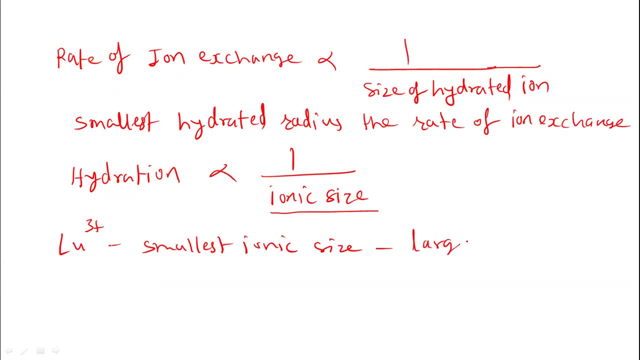 so it is having largest hydrated radius. largest hydrated radius, okay, or largest hydrated size. it means that lutetium tripositive ion it is having the smallest ionic side, so it is hydrated mostly because water molecules get combined with this lutetium tripositive ion very easily, because it is having the smallest ionic. 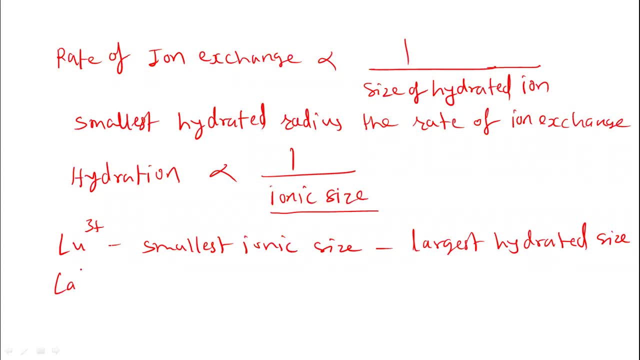 size and lanthanum tripositive ion which is having largest ionic size. largest ionic size. okay then it is having smallest hydrated radius, smallest hydrated size. this is because it is having the largest ionic size- lanthanum tripositive- and we know that hydration is inversely proportional to the ionic size. 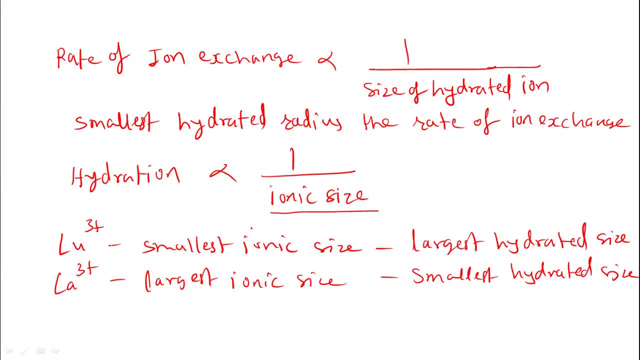 so according to this we can say that the lutetium tripositive ion it is having the largest hydrated radius, largest hydrated size and lanthanum tripositive ion it is having the smallest hydrated size, so rate of the ion exchange it is greater in case of. 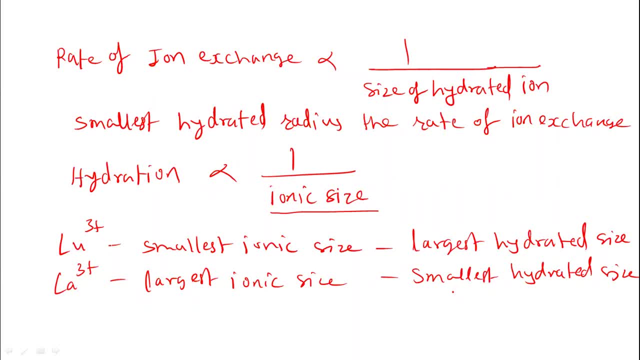 lanthanum tripositive ion. first because it is having the smallest hydrated size, so rate of ion exchange is greater. in case of rate of ion exchange. rate of ion exchange is greater. rate of ion exchange is greater in case of: in case of lanthanum 3 plus ion, lanthanum 3 plus ion and rate of 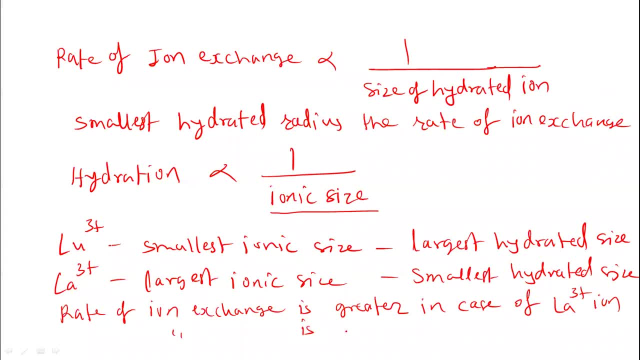 ion exchange is less or least in case of: in case of lutetium tripositive ion. okay, because lanthanum tripositive ion it is having smallest hydrated radius and lutetium tripositive ion it is having largest hydrated radius. so as the rate of the ion exchange will, 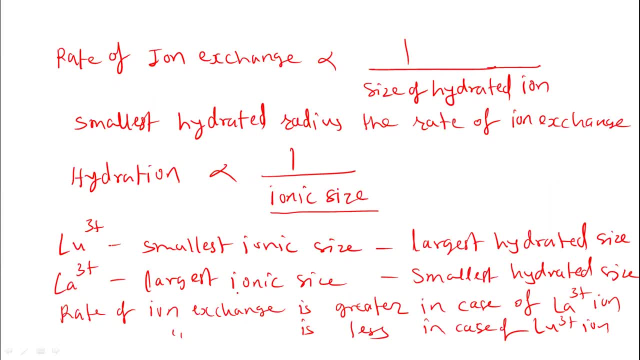 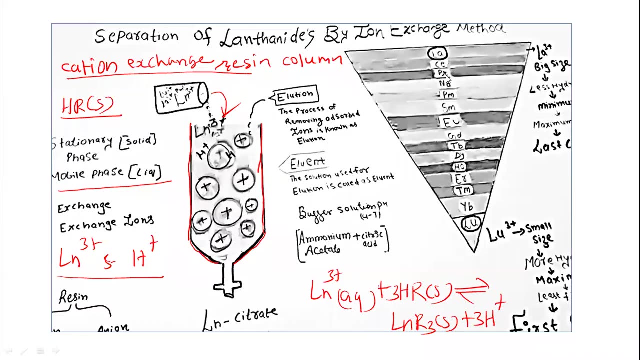 be greater for lanthanum tripositive ion. so it will be. it will exchange first with the resin column and as the rate of the ion exchange will be less in case of lutetium tripositive ion, so it will exchange last with the resin column. so you can see here in this diagram. 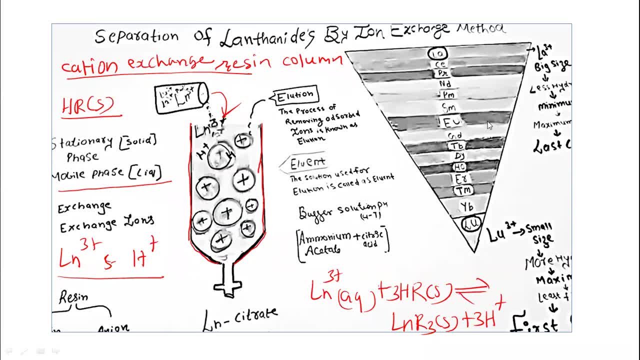 okay, in the resin column, the lanthanum tripositive ion. it is at the top of the column. okay, it is at the top of the column, see, because it is having the largest uh uh. it is having the smallest hydrated radius and largest ionic size. then second, which is exchange, it is cerium tripositive ion. 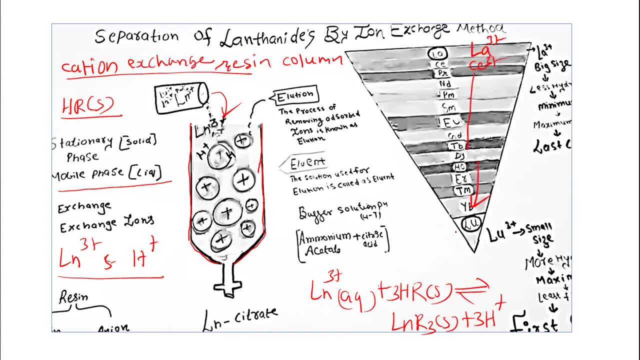 and last, which is exchange. it is lutetium tripositive ion because it is having the largest hydrated radius. okay, so you can see here, lutetium tripositive ion, it is having the small size, more hydrated, so rate of the ion exchange will be less here. lanthanum tripositive ion, which is 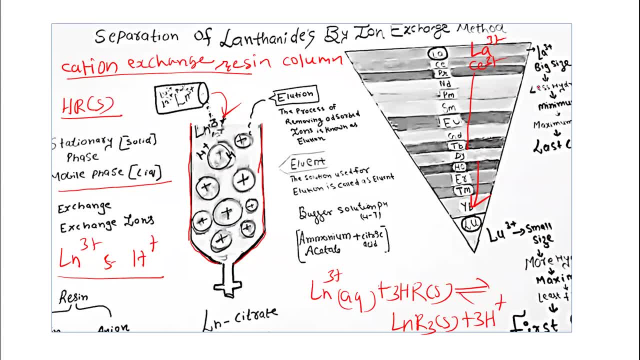 having bigger ionic size, less hydrated radius, so it is having uh largest rate of the ionic change. so according to this we can say that lanthanum tripositive ion it is exchanged first with the region column and it is remains at the top of the column. 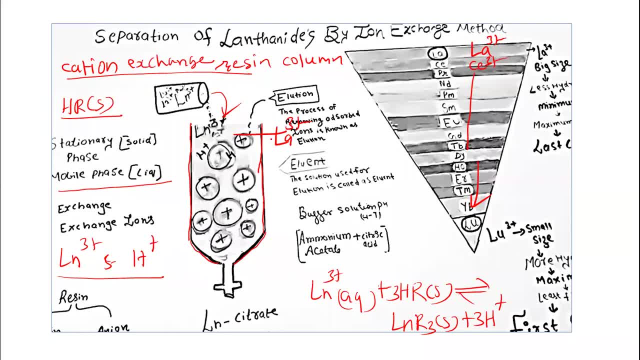 so in this way, one by one, all the lanthanon ions are attached with the resin. all the lanthanum ions are exchanged with the region. okay, so this is very important here, because there are 15 lanthanum ions and we know that according to the lanthanum contraction. 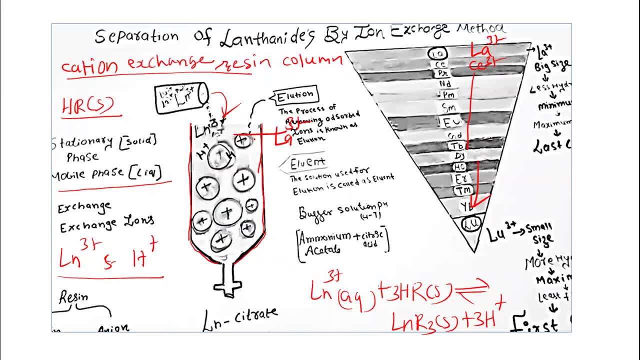 contraction and the second second effect of the lanthanum: contraction. marginal variation in the size causes minor variation in the properties. it means the ionic size of the lanthanum ions are not same to same. so lanthanum tri positive i it is having the largest ionic size and smallest. 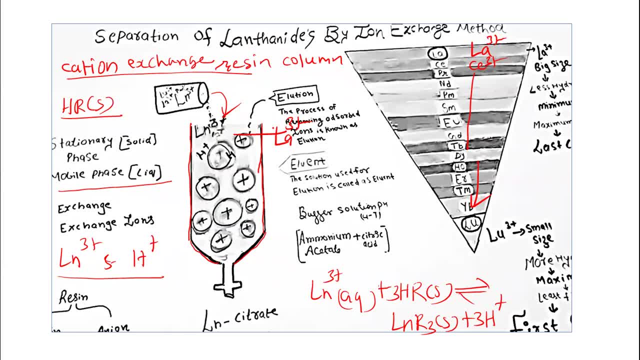 hydrated radius, so it is going to be exchanged first with the region column and lutetian tri positive ion. it is having smallest ionic size and largest hydrated radius, so it is exchanged last with the resin column and in this way all the lanthanum ions are exchanged with the resin column. 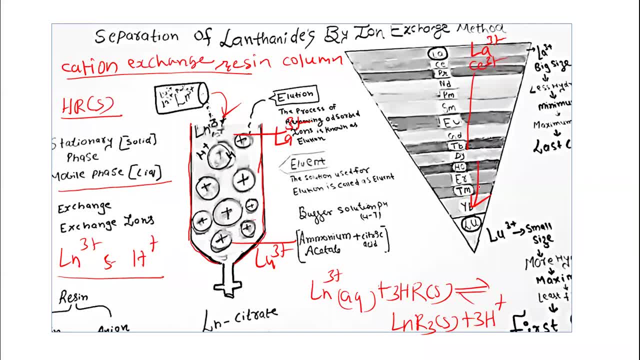 they are going to be attached to the. They are going to be absorbed on to the resin column. So the lanthanum ions now are bind with the resin column. So in this case lanthanum, tri positive ion, the first ion, first lanthanum. 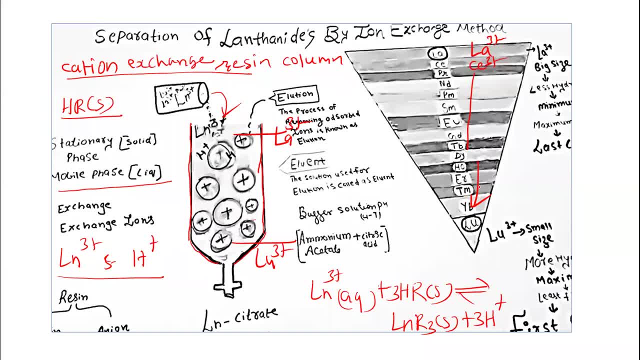 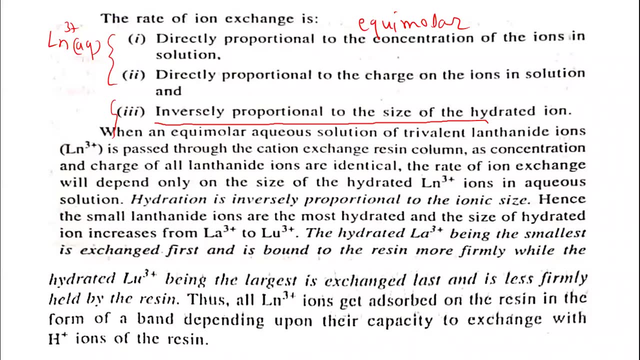 first lanthanum, that will be exchanged first with the resin column And last it is lutetium tri positive ion. So exchange process is takes place here. Exchange process is takes place here- So again that will be explained here- When we are adding the equimolar aqueous solution of the trivalent lanthanum ions. 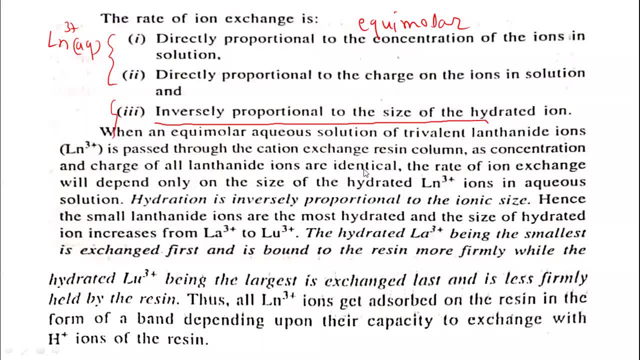 it is passed through the cation exchange resin column. We know that concentration and charge of all the lanthanum lanthanides are same. So rate of exchange: The rate of the ion exchange depends upon the size of the hydrated lanthanum ions in aqueous solution. 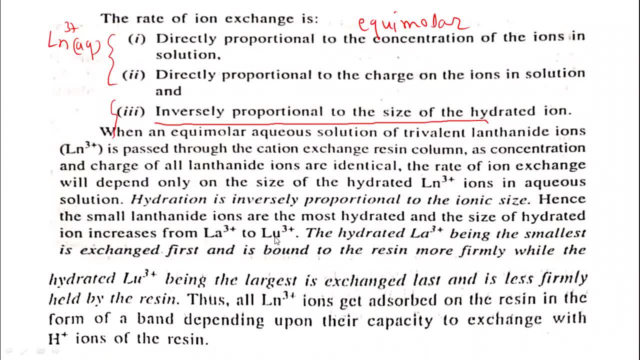 So the lutetium tri positive ion: it is the largest, It is having the largest hydrated radius, So it will be exchanged last. And lanthanum tri positive ion: it is having the smallest hydrated radius, So it will be exchanged first and it is bound to the resin more firmly, more strongly. 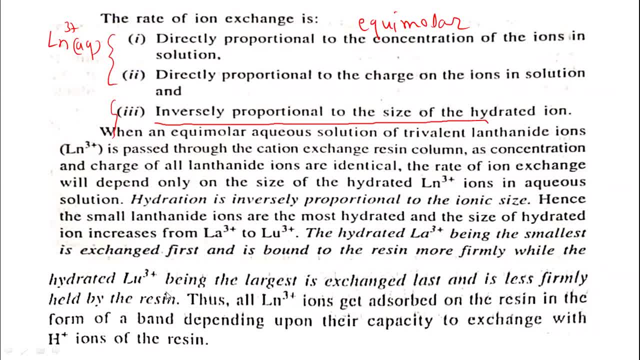 While the hydrated lutetium tri positive ion being the largest, is exchanged last and it is less firmly held by the resin. So in this way, one by one, all the lanthanum ions get absorbed on the resin column in the form of the bag. 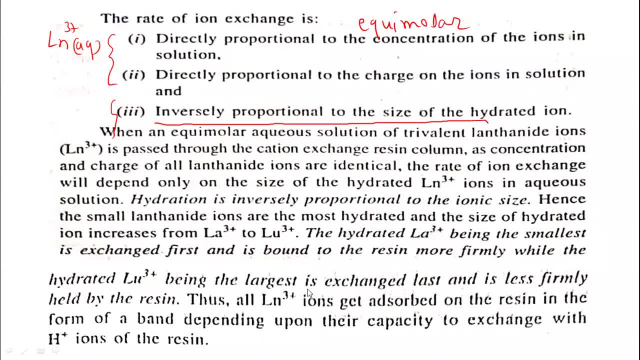 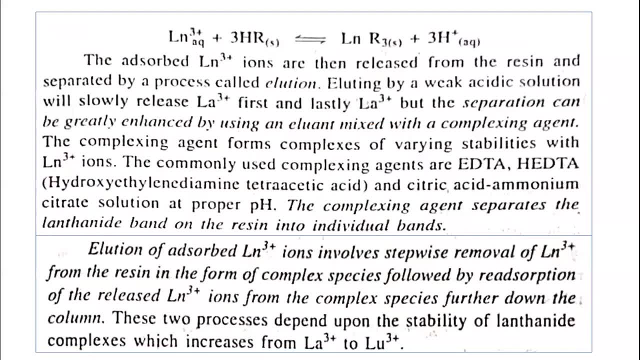 Their individual bands are supposed to be created in the resin column. Their individual bands are supposed to be created with the resin column. Now you can see this diagram here, One minute. See this. So this is the first step. Already we have explained this. 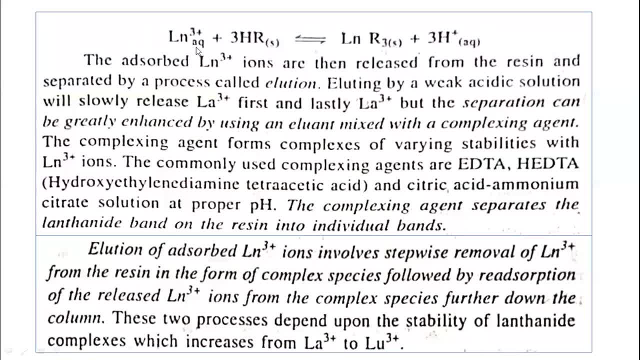 When we have equimolar concentration of the lanthanum ion in the resin column. So exchange process will be takes place here And lanthanum ions get attached with the resin column. So this is the first step that has been already explained by us. 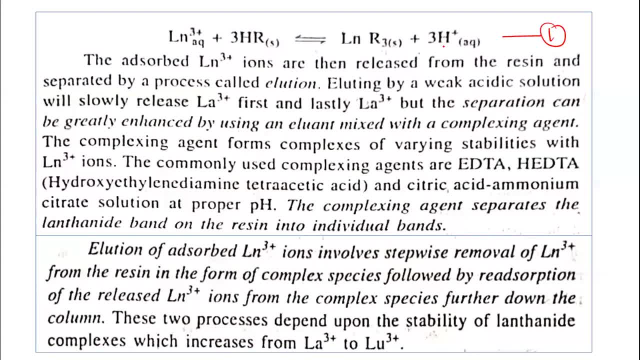 And hydrogen ions are free. Now we want to separate the lanthanum from each other. We want to collect the eluent of the lanthanum ions. We want to collect the fraction of the lanthanum ions. Now they are going to be attached to the resin column in this step. 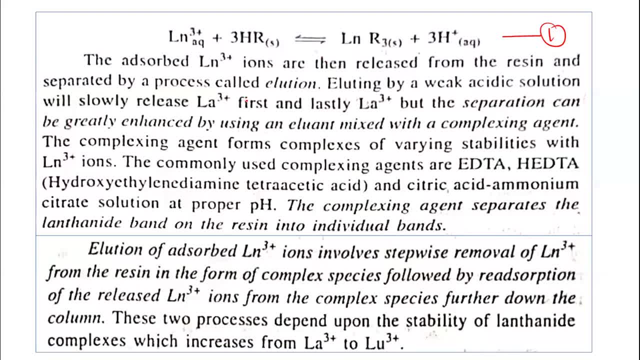 But how they can release now from the resin column. So the absorbed lanthanum ions are then released from the resin And separated by a processor, And separated by a process called elution process, Because we want to collect the 15 lanthanum ions. 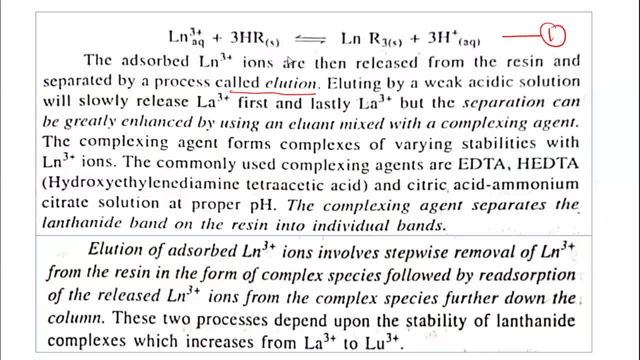 We want to separate them. We want to collect the 15 lanthanum ions. So how they are now separated from each other. So the absorbed lanthanum ions are released from the resin And separated by a process It is called as a elution process. 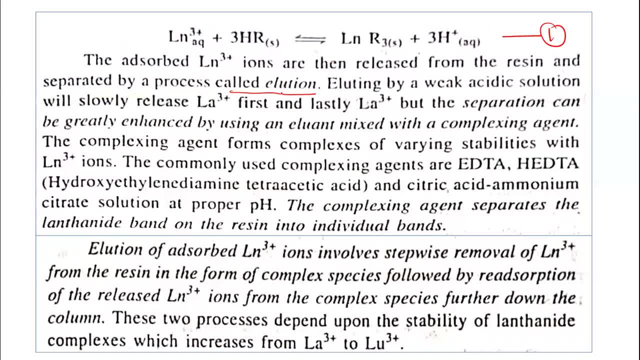 Next step. it is the elution process. So we have to add the eluting agent. in this case, We have to add the eluting agent or eluting solution In the resin column. In the resin column, That is weak acidic solution. 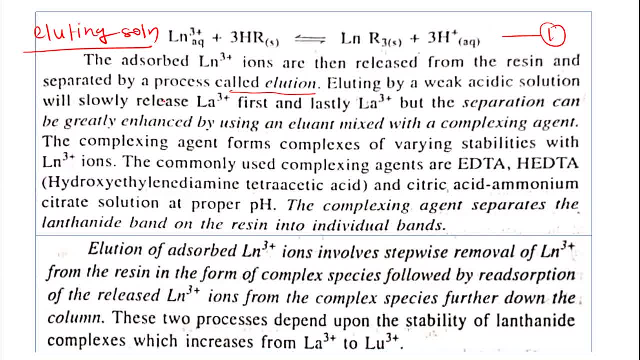 We have to add once again the acidic solution in the resin column, So releases. We will slowly release lanthanum tri positive first, And lastly, we will release slowly first lutetium tri positive. Why lutetium? Because it is less firmly held with the resin column. 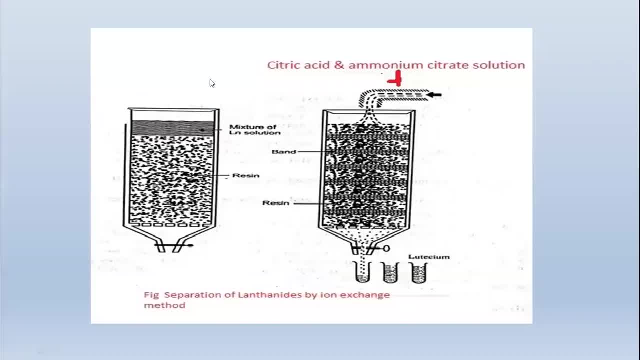 You can see This lutetium tri positive ion which is exchanged last. Once again, I would like to show in this diagram, See See: Lutetium tri positive ion. it is exchanged last year. And lanthanum tri positive ion. it is exchanged first with the resin column. 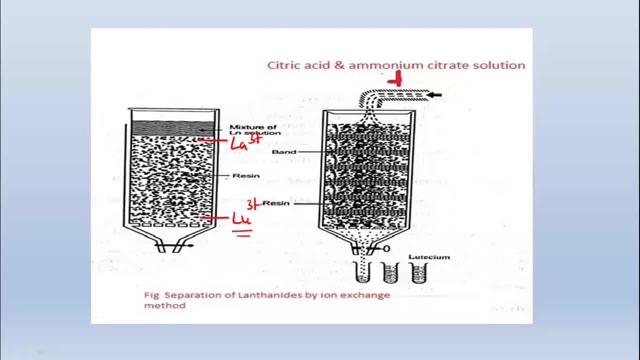 So lutetium tri positive ion. it is less firmly held with the resin column And lanthanum tri positive ion. it is strongly held with the resin column Because rate of the ion exchange will be Greater here in case of the lanthanum tri positive ion. 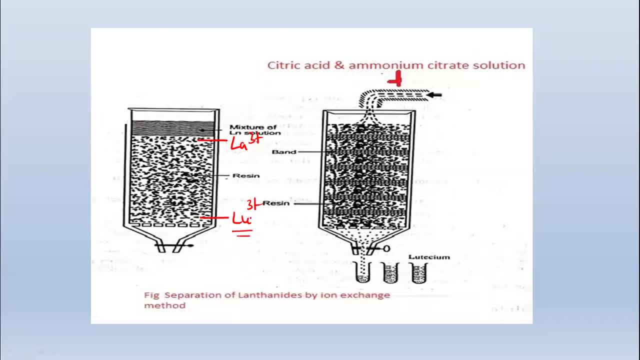 And rate of the ion exchange. it is minimum here In case of the lutetium tri positive ion. So in the first step the lanthanum ions are attached to the resin column. The lanthanum ions are attached to the resin column. 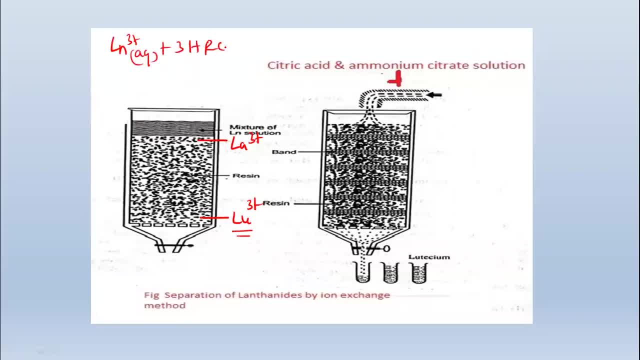 You can see we already showed this. This is the first step. The lanthanum ions get bind with the resin column, So the lanthanum ion, which is bind less firmly with the resin column. Now in the second step, By adding the eluent. 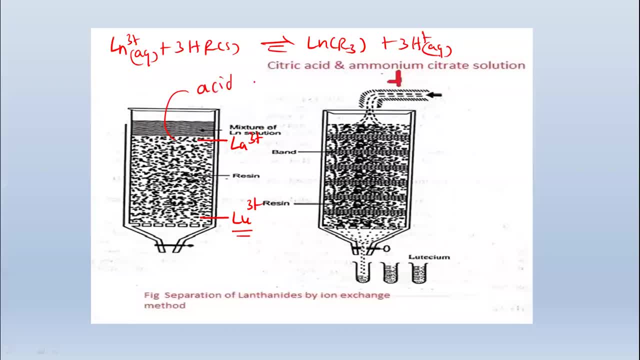 Or acidic solution, Acidic solution of Suppose, hydrochloric acid solution or sulfuric acid solution. we are going to add here What happens. The lanthanum ions are released from the resin. How they are released: The lanthanum ions, which are less firmly held with the resin. 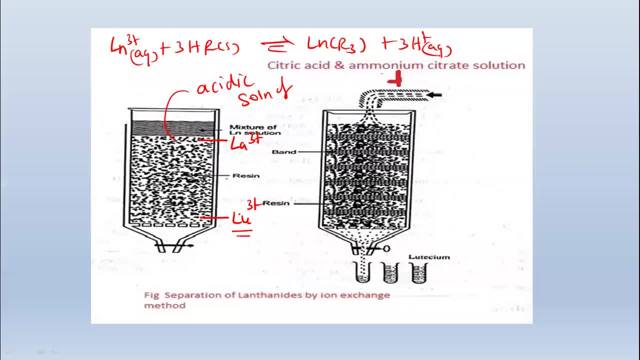 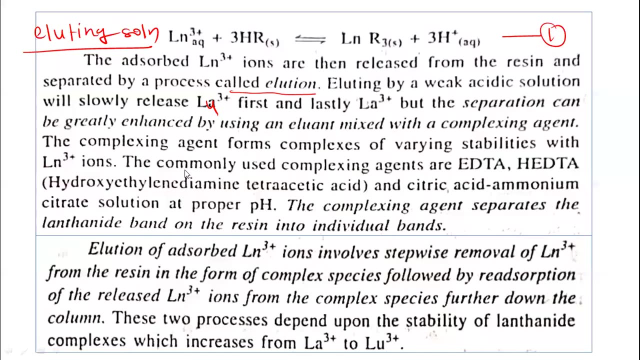 They are released first. So lutetium tri positive ion is released first, Then ytterbium, Then thulium And last it is lanthanum tri positive ion. So they are released first With the resin column. This is the second step which takes place here. 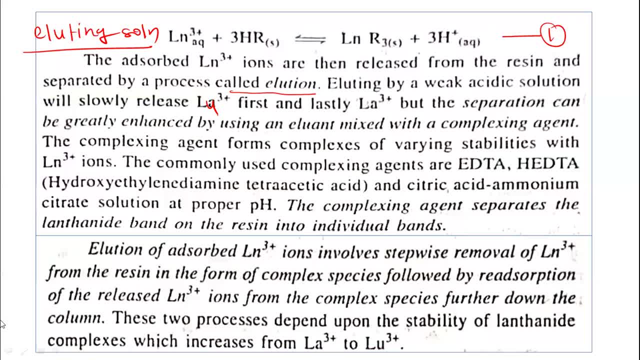 Okay, This is the second step. But actually in this case, acidic solution- it is not sufficient to create the individual bands of the lanthanum ion, Okay, So therefore we have to add a complexing agent here In the separation of the lanthanum ions. 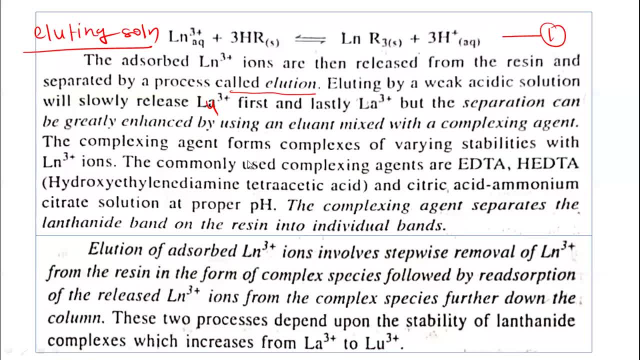 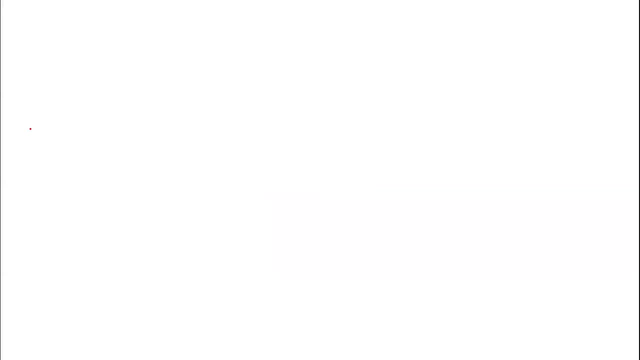 Complexing agent playing a very important role in the separation of the lanthanum ion. Only acidic solution, it is not sufficient. Only acidic solution it is not sufficient to create the individual bands of the lanthanum ions. So therefore we have to add the eluent mixture with complexing agent. 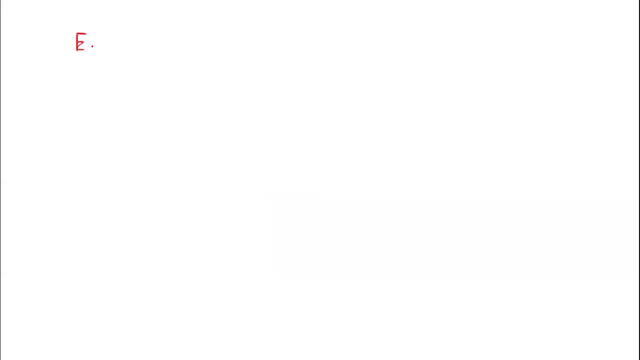 Eluent mixture with complexing agent, Complexing agent: Complexing agent In the resin column. So in this case, the mixture of ammonium citrate, Ammonium citrate and citric acid is added. Mixture of ammonium citrate and citric acid is added into the resin column. 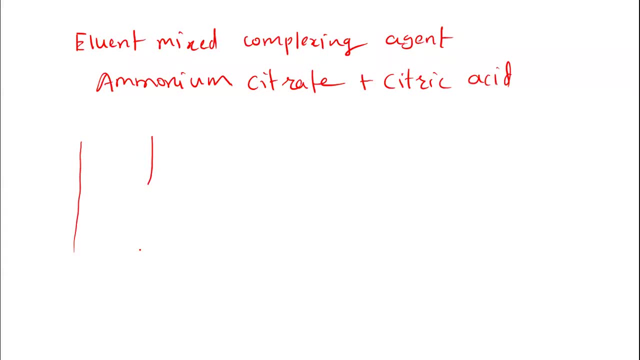 Okay, Diagram- once again: Mixture of ammonium citrate citric acid. it is added into the resin column. Okay, So at the bottom, lutetium tri-positive ion is there And at the top, lanthanum tri-positive ion is there. 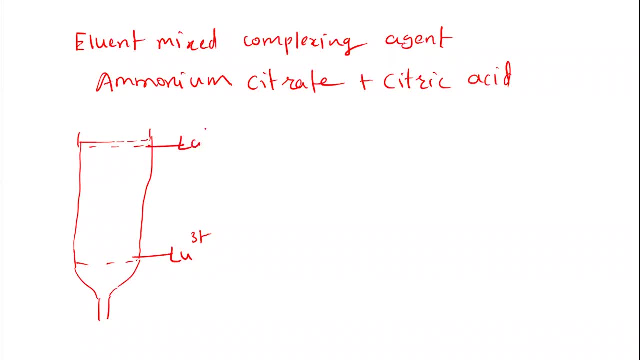 Okay, In the first step, And due to the addition of the acidic solution, proper separation of the lanthanum is not takes place. So therefore we have to add the mixture of ammonium citrate and citric acid in the resin column. So, due to the addition of this, individual banks of the lanthanums are created in the resin column. 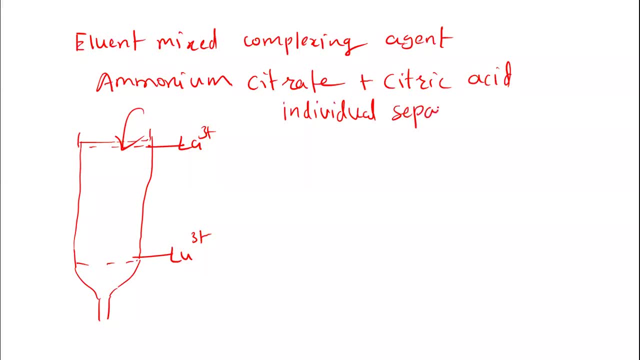 Individual separation of lanthanum ions. Individual separation of lanthanum ions are takes place. Now, when we are adding the ammonium citrate and citric acid in the resin column, what happens First of all? once again, right here, the first step, that is, addition of lanthanum solution in the resin column. 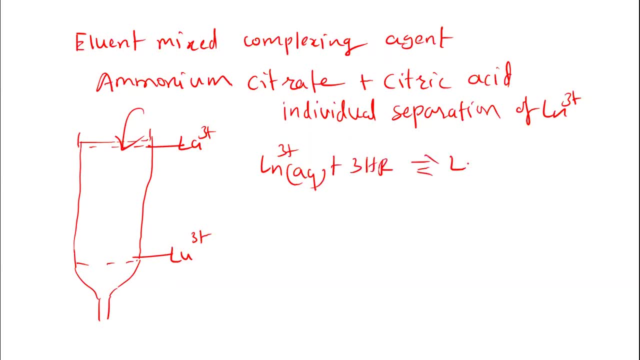 And this equilibria is established here. Lanthanum ions get attached to the resin column. Okay, Now in the second process the eluent mixture with complexing agent should be added. Only eluent is not sufficient. Eluent means which releases the lanthanum ion from the resin column. 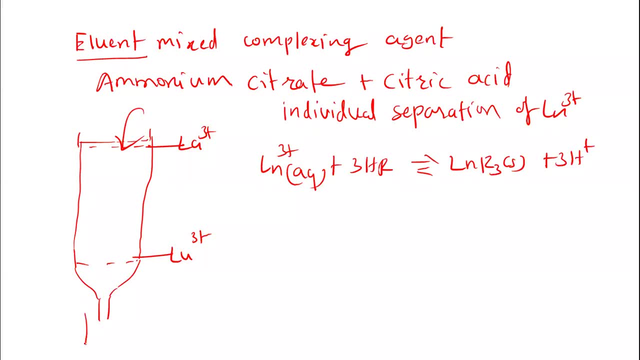 And we are collecting the fractions here of that particular lanthanum ion. We are collecting the fractions one by one. So when we are adding the eluent mixture with complexing agent, Then it will create the individual banks in the resin column. Individual banks are formed here like this: 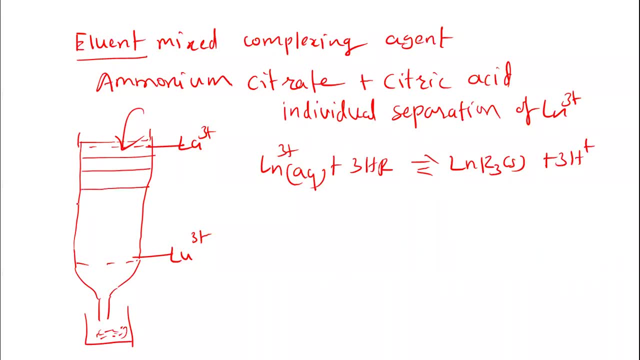 Individual banks of the lanthanum ions are formed in the resin column And one by one, we can collect that fraction. Okay, And the fraction which is here at the bottom, it belongs to the lutetium tri positive ion. And the fraction which remains at the top, it belongs to the lanthanum tri positive ion. 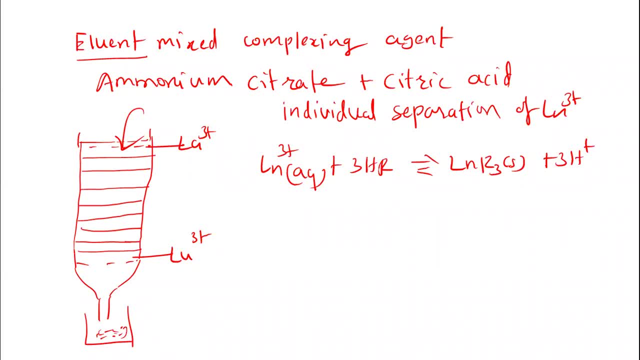 But let us see what process takes place here. So this is the first step. So this is the first step. The lanthanum ions are attached to the resin column. Now we want to separate them, We want to release them from the resin column. 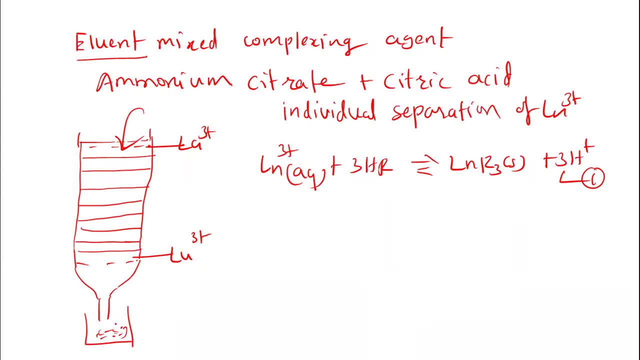 Because we want to collect the fraction. That process, it is called as the elution process. Therefore, we are adding the mixture of ammonium citrate and citric acid. Citric acid, it is a complexing ligand, It is a bidentate ligand. citric acid. 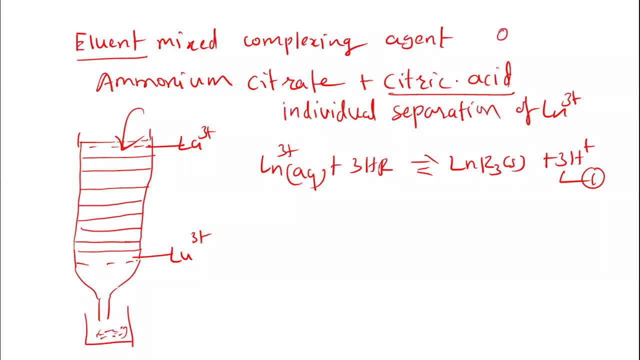 Oxygen is a donor atom there in the citric acid. I think So when we are adding this mixture, ammonium citrate and citric acid, what happens? The ammonium ions, which are present into the ammonium citrate. they react with this resin column. 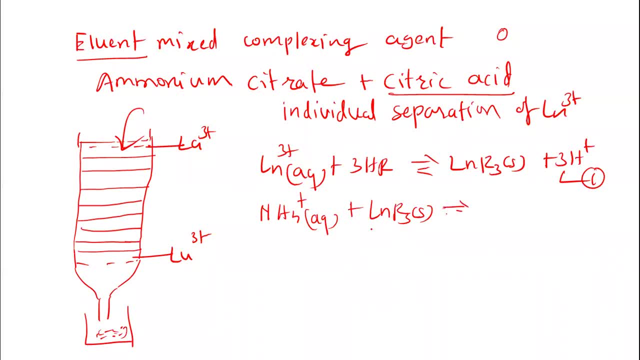 And what happens here? Once again, the cation exchange process takes place. Ammonium ions are cation, Lanthanums are cation, Lanthanums are cation. So there is a formation of this. Okay, There is a formation of this process. 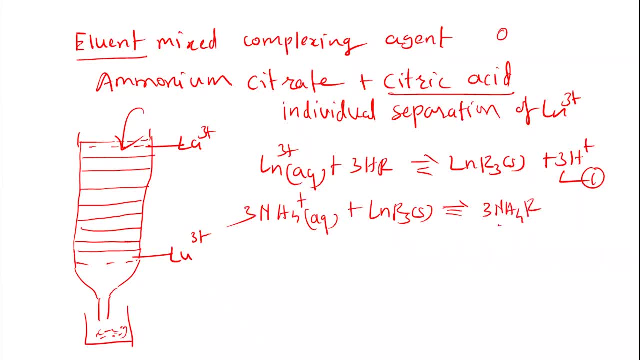 Rice, NH4, R, So ammonium ions get attached to the resin column, And now lanthanums are separated from the resin column. Okay, Lanthanum ions are now free from the resin column. So once again here, cation exchange process will take place. 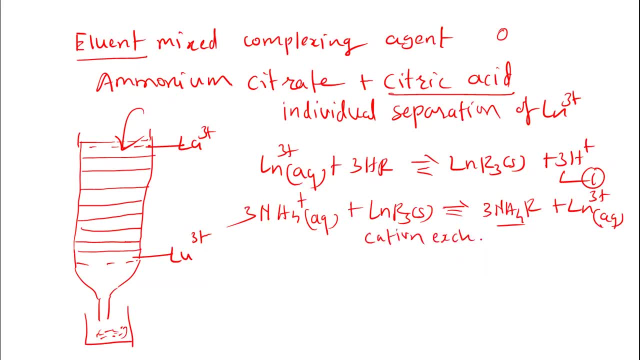 Cation exchange process takes place here. Okay, The cation ammonium ions get exchanged with the lanthanum ions. So in this case, what happens? The lutetium tri-positive ion. it is released first from the resin column because it is less firmly held with the resin column. 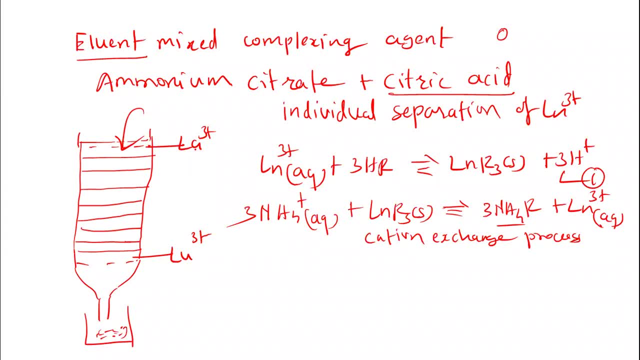 And lastly the lanthanum tri-positive ion. it is released from the resin column. So if suppose lutetium tri-positive ion, it is released first, Then it is going to form the complex with the citrate ion. It is going to form the complex with the citrate ion. 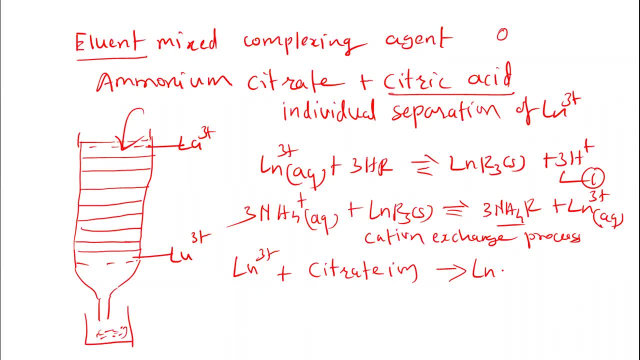 And this lanthanum citrate complex is formed here. Lanthanum citrate complex, It is formed here. All the lanthanum ions are going to form the complex with the citrate ion. All the lanthanum ions are going to form the complex with the citrate ion. 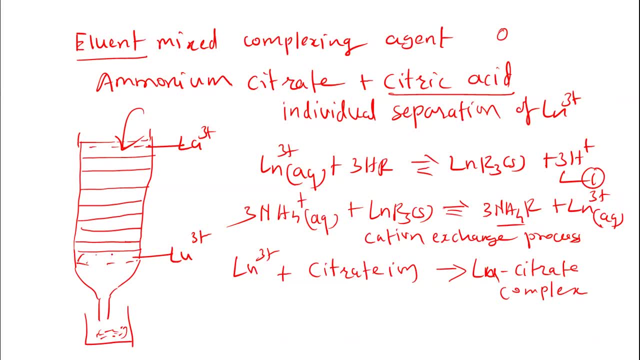 So suppose now this is the complex of the citrate ion of the lutetium, Then complex of the ytterbium here, And it is here the complex of the lanthanum tri-positive ion. So in this way lanthanum ions are separated from each other one by one. 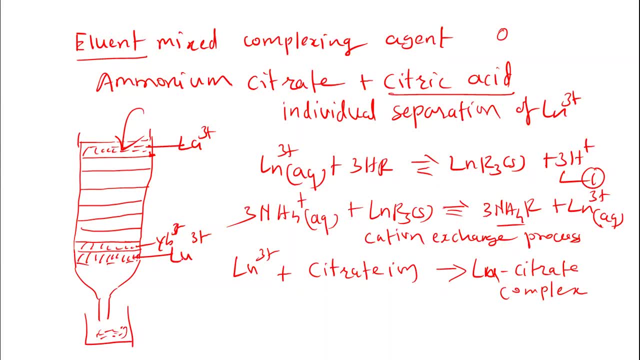 And bottom portion it belongs to the lutetium tri-positive ion And topmost portion it belongs to the lanthanum tri-positive ion. Now, these ions are associated with the ligand means. complex is there? Then we can collect the fraction here. 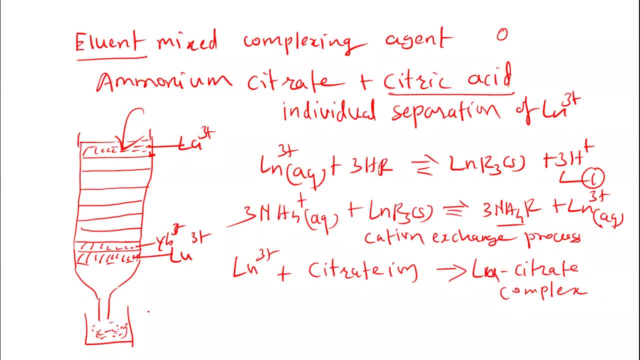 We can collect the fraction here. So, first fraction which is collected, it is the lutetium. Second fraction which is collected, it is ytterbium. Third fraction which is collected, it is supposed to be thulium. reverse order. 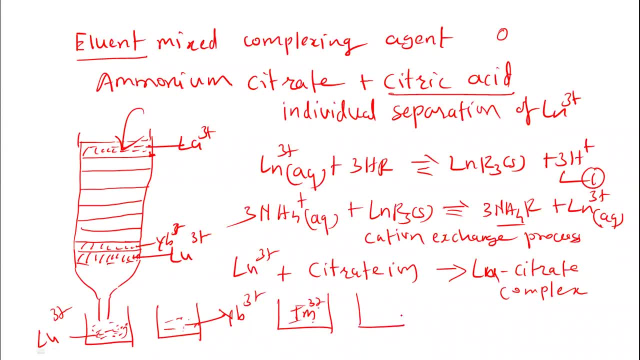 And last fraction, or the last lanthanum ion which is eluted, that is, the lanthanum tri-positive ion. So in this way the lanthanums are separated in the reverse order. First, the last lanthanum ion. it is lutetium tri-positive ion because it is at the bottom of the resin column. 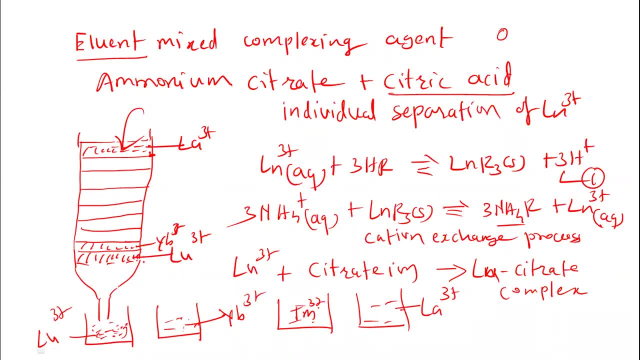 So it will be eluted first. its fraction will be collected. Its fraction will be collected here. With the help of this top quark, we can collect this fraction. Lanthanum ions are individually separated from each other. Their individual bands are created. 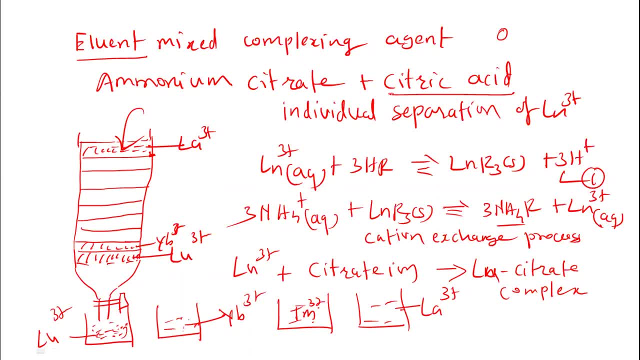 Why their individual bands are created? Because, due to the addition of this ammonium, citrate and citric acid, The ammonium ion replaces the loosely bound lanthanum from the resin. That is lutetium first And that lutetium tri-positive ion is going to form the complex with the citrate ion. 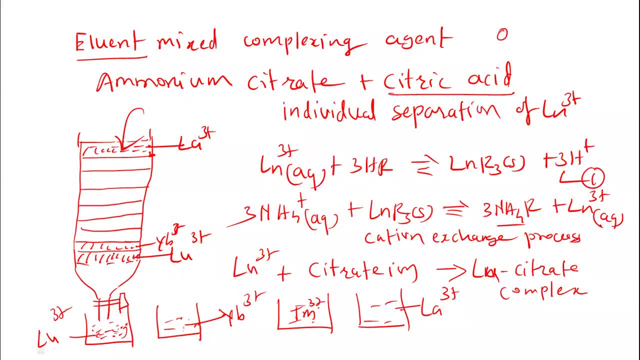 So lutetium citrate complex is formed here, So its bands are created here, Then ytterbium, Then thulium, Then erbium, Like that, Then dysprosium- Sorry, holmium, dysprosium, gadolinium, in the reverse order. 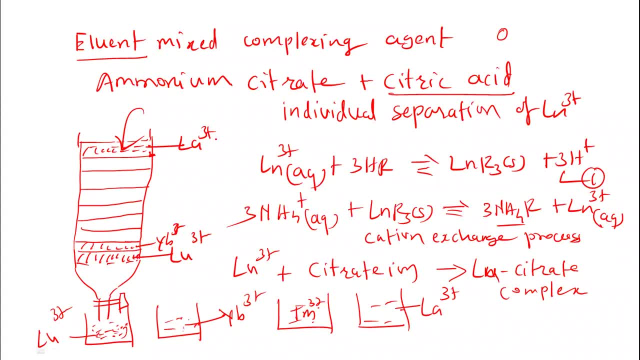 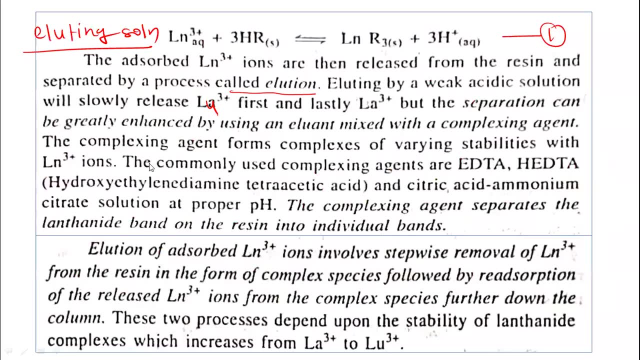 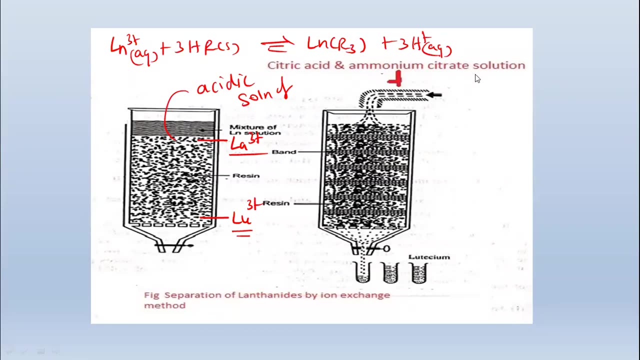 And at the top position that is the lanthanum tri-positive ion. So there is a creation of the individual bands in the resin column. There is a creation of the individual band You can see in this diagram. Okay, Citric acid, ammonium, citric solution. 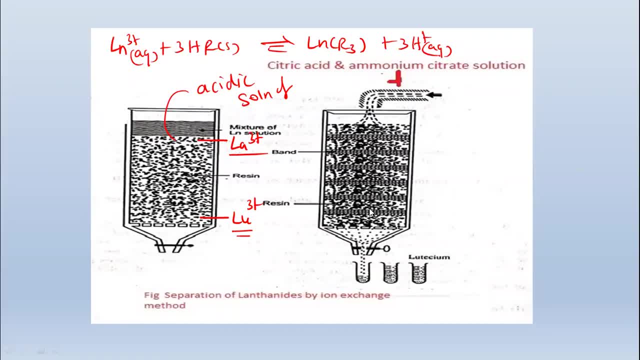 It is added here. You can see how the individual bands are created here in the resin column. The individual bands are created in the resin column here. So you can see this is lutetium, that will be collected first, Then ytterbium. 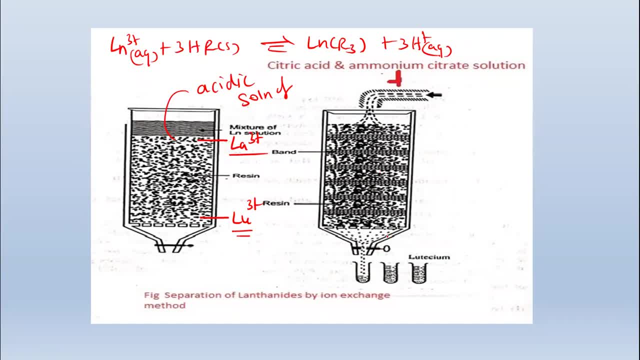 Now then this is thulium. Okay, So you can see in this diagram, because lutetium it is at the bottom and lanthanum it is at the top. So first lanthanum ion, which is separated, it is the lutetium tri-positive ion- and last,